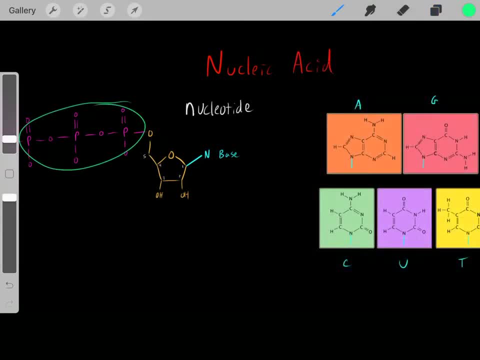 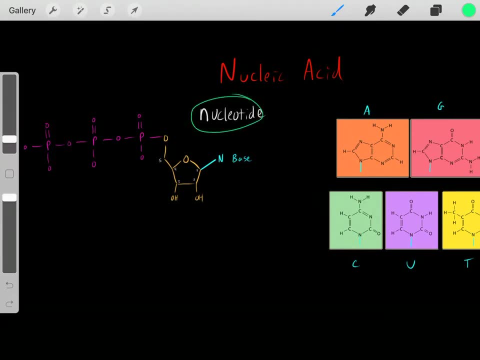 it. So we phosphorylate it, adding these phosphate groups. Now, once we added these phosphate groups, now we have a nucleotide, Now we formed a nucleotide. So nucleotide is just a ribose carbohydrate with a nitrogenous base on carbon 1, and these phosphates on this oxygen, on carbon 5.. 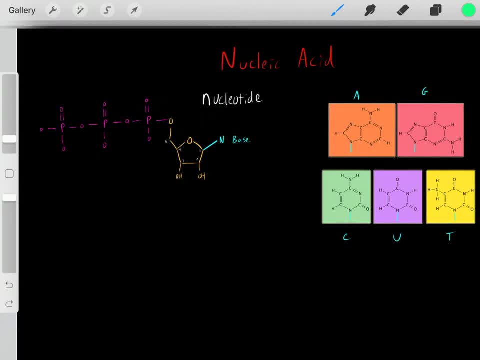 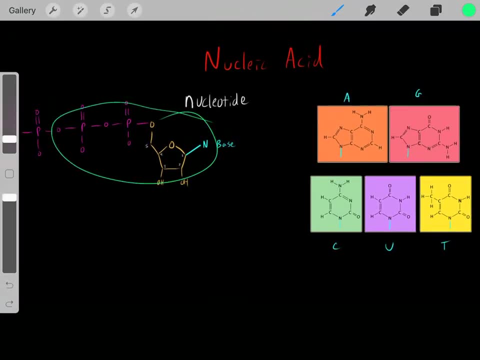 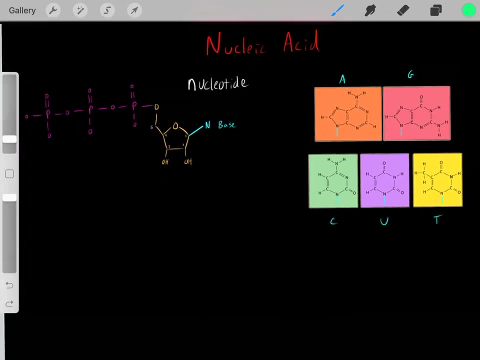 And again, we can have a triphosphate nucleotide, We can have a diphosphate nucleotide in a monophosphate nucleotide, depending on how many phosphate groups we have. But now we have a nucleotide And these nucleotides are the building blocks for RNA, for an RNA strand. So again, 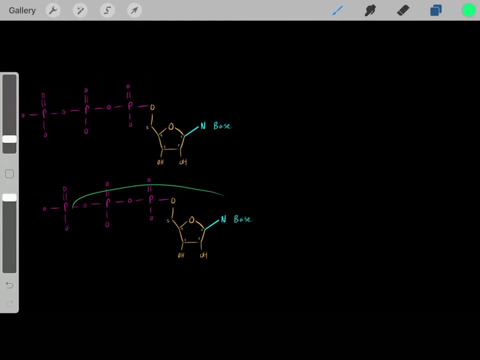 let's do an example. Let's say: now we have a second nucleotide, So now we have these two nucleotides, Now we can add these nucleotides together, We can form covalent bonds between these nucleotides. And how do we do that? Well, essentially, this carbon, I mean this oxygen on. 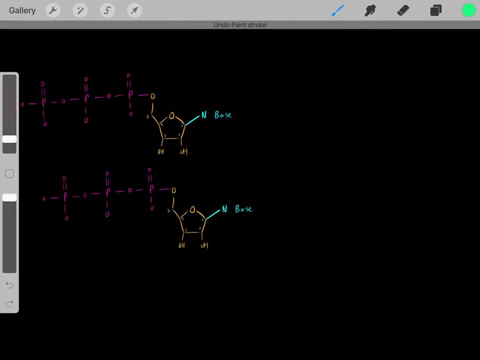 this carbon 3, we take this oxygen with its lone pairs of electrons and it can act as a nucleophile. It nucleophilically attacks this phosphate. So it nucleophilically attacks this phosphate forming a bond. And once we form that bond, eventually what we do is we break this bond. 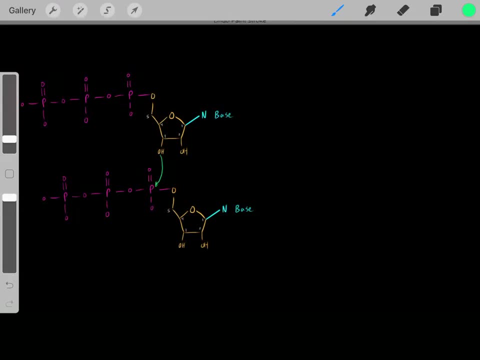 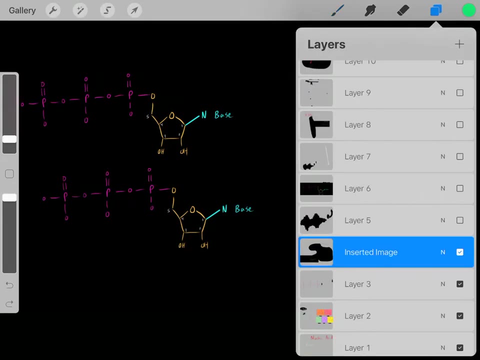 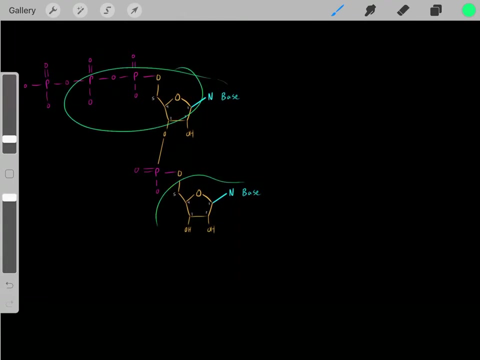 This bond is broken and these electrons form this oxygen. So notice what we're doing. We're forming a bond and we're breaking a bond and this guy would just float away. So if we did that, form that bond and then we broke that bond, Now we covalently linked these two nucleotides. 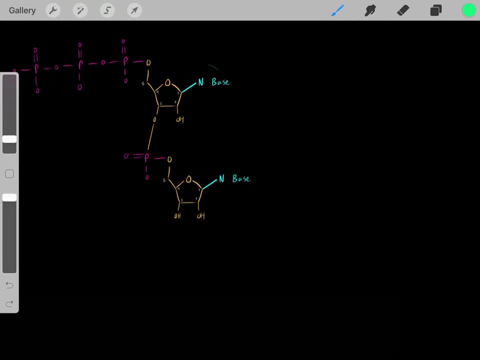 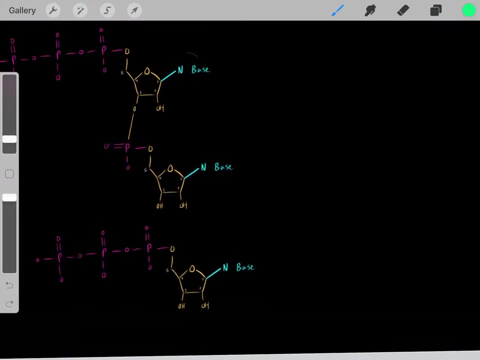 together with one of these phosphodiester linkages. So we can go a step further. Now we can take another nucleotide, Now we have another nucleotide and now we can add another nucleotide to that same mechanism. This oxygen attacks. When it attacks this bond, breaks these electrons. 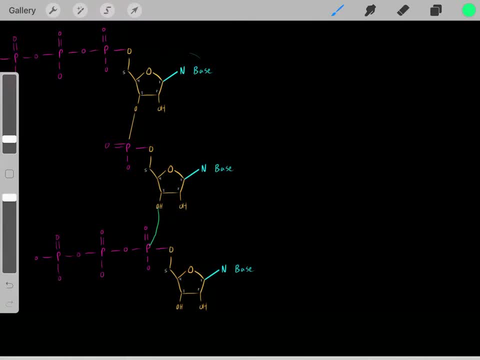 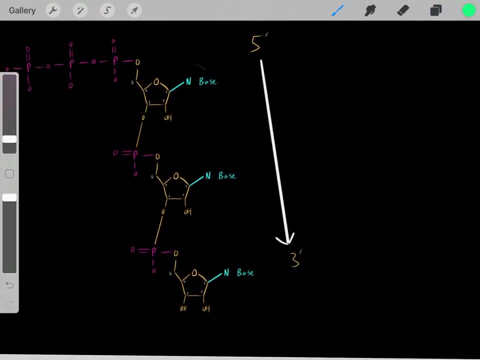 fall on this guy and this part floats away. So we form a bond and we break a bond. So if we did that again now, we would add another nucleotide. So again we can take another nucleotide and we can. that's actually how we form these strands of RNA. And again, you might've learned in a genetics. 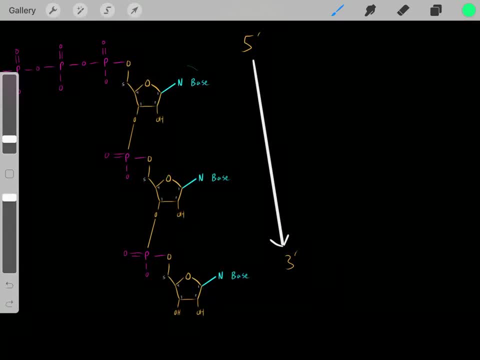 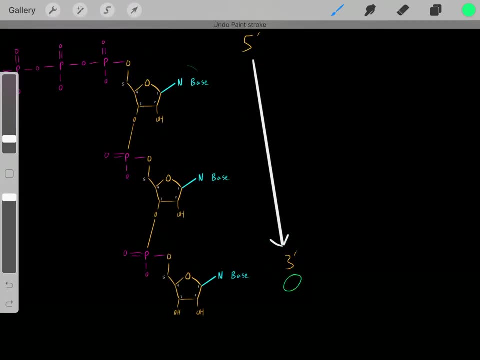 class, When we create strands of RNA and DNA. how do we do them? We go from five to three. It's on, we go from the five prime end to the three prime end And it's on this three prime end where we keep on adding new nucleotides. And that's why- because remember, this was carbon five. 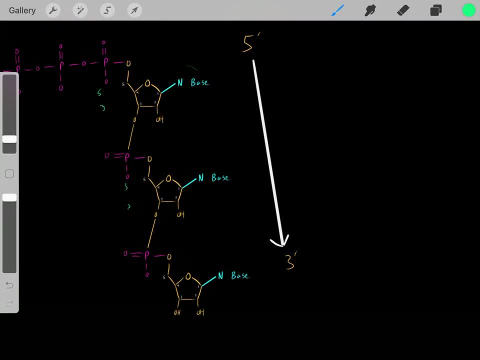 this was carbon three, So five, three, five, three, five, three, et cetera. So we're going in this direction, We're adding nucleotides to the five, three, five, three, et cetera. 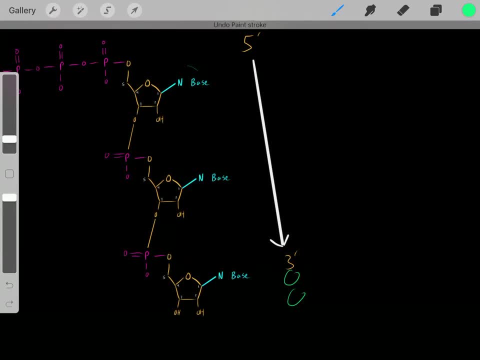 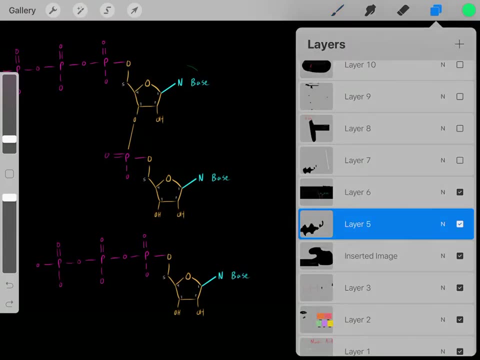 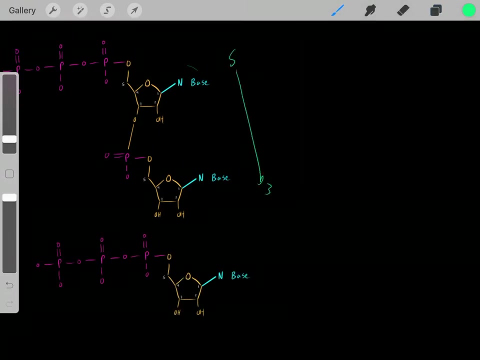 To the three prime end. we're adding nucleotides to this three prime end And that's why we always go five to three, Cause remember what happened, Remember we, we added it here, We, we, essentially we, we added this guy, We, we again remember five to three, and then it's on this three prime end. 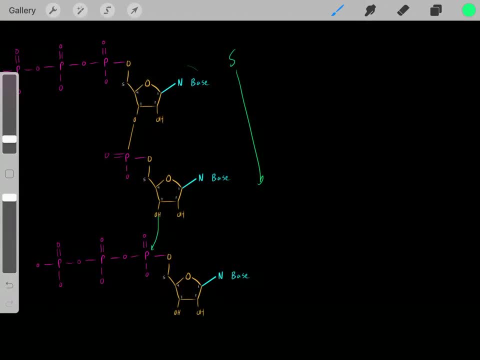 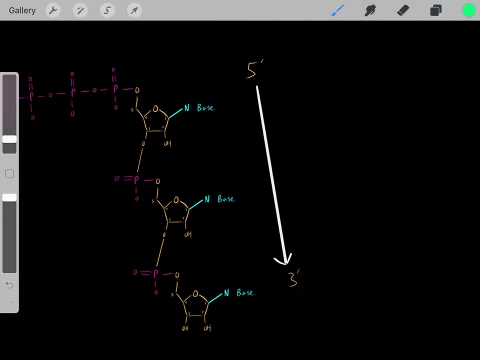 where we add more, Cause it was this three prime end where we form that bond, adding the new nucleotide. That's why we added it on this three prime end And that's why we always go five to three. But again, now we formed one of these nucleotides. I mean now we formed one of these poly nucleotides. So 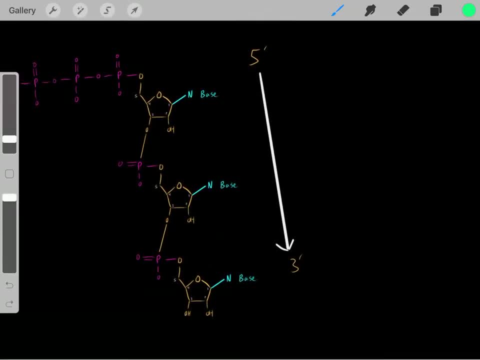 now we have a mini strand of RNA, And now we know so this is a strand of RNA. For example, when we make mRNA, even though we do more modifications, it essentially this is what it looks like It's. it's these, these nucleotides linked together. So, again, this is a strand of. 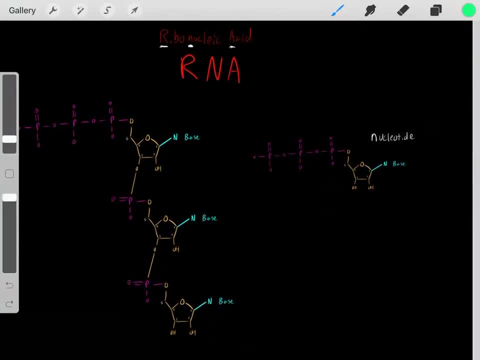 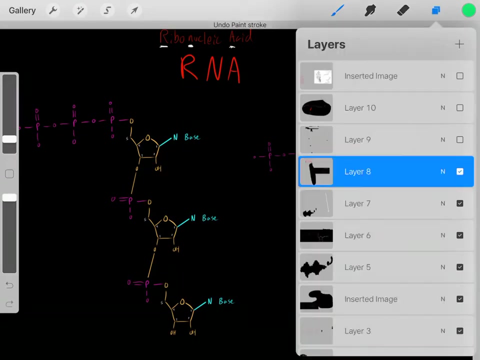 RNA, which is made out of these nucleotides, but we also know we have DNA. So what's the difference between this RNA, these, this RNA strand with DNA? Well, notice this oxygen on carbon two, these, these oxygens on carbon two. So, again, instead of having an oxygen on carbon two, we just have a. 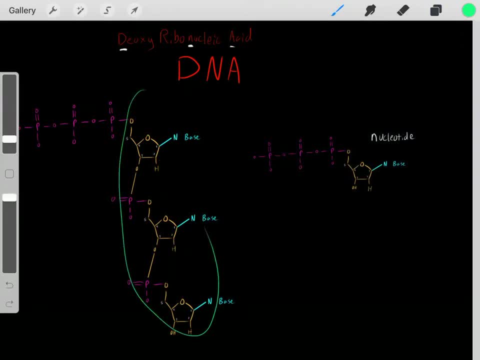 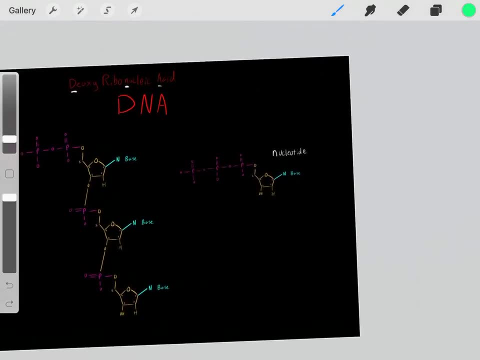 hydrogen. If we just have a hydrogen now we have a strand of DNA. So that's the difference. These DNA strands are made out of these nucleotides with the hydrogen on this carbon two. So if we're using, if the nucleotide has a hydrogen on carbon two, it's used to create DNA. However, this 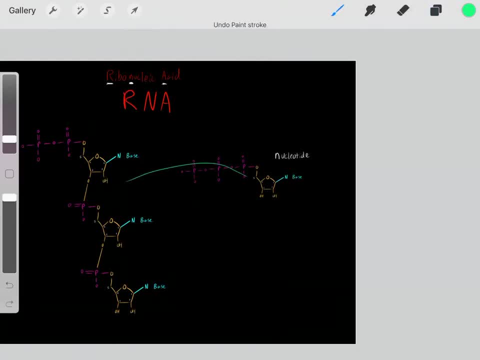 carbon two instead has a hydroxyl, then that's used to make RNA. but that's the difference: If we have hydroxyls, that's RNA, If we have hydrogens, that's DNA. So again, and we know.